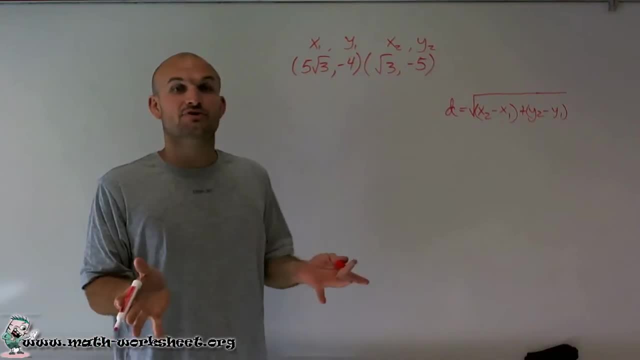 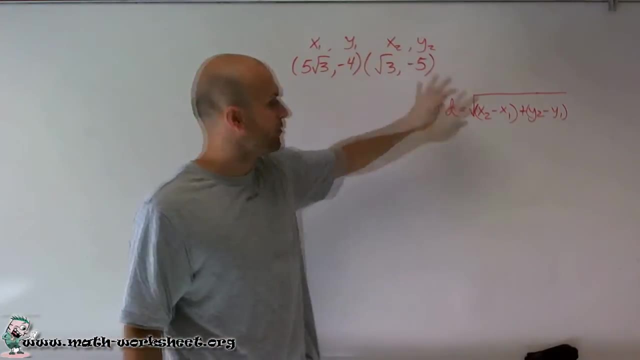 So the only reason why we just use the 1 and 2 is just to differentiate between the two coordinate points. So now what I'm going to do is I'm simply just going to evaluate by plugging in my coordinate points into the equation. 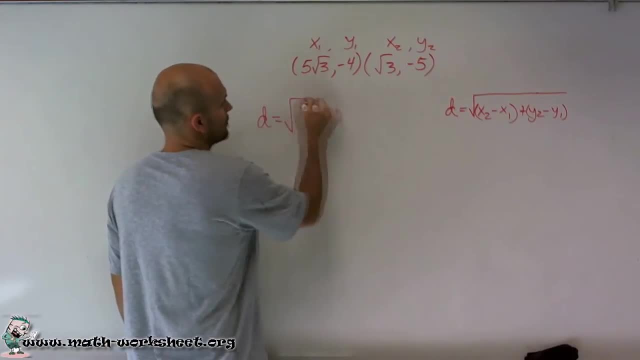 So I'll just rewrite it here. So I'll say: the distance is equal to the square root. x2 is square root of 3, minus 5, square root of 3.. And then we have that's in parentheses. oh, I'm sorry. 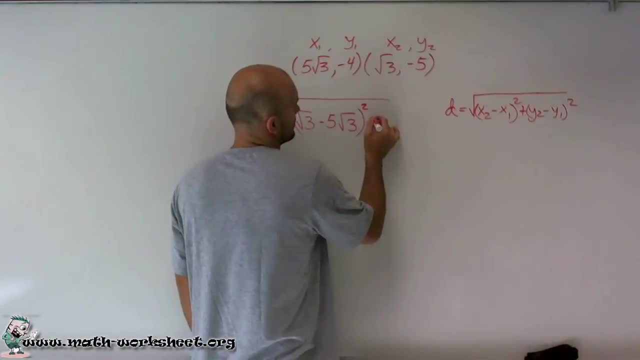 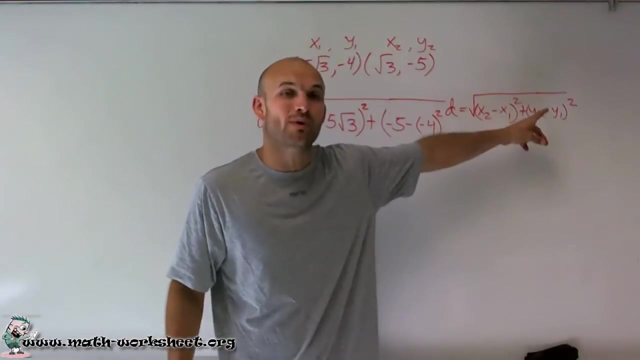 squared: plus y2,, which is negative, 5, minus y1,, which is negative, 4, squared. So it's a really important one. I'm sorry, I just kind of a little forgot I was writing it down. Make sure you square it. 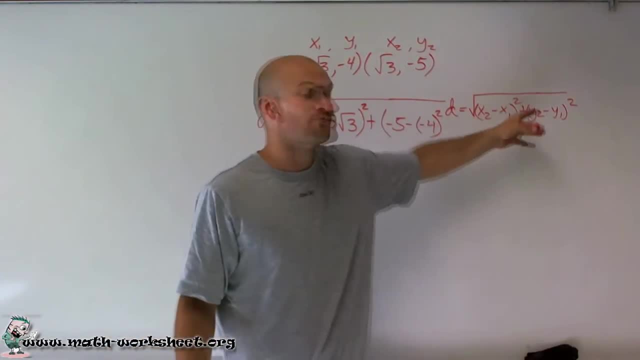 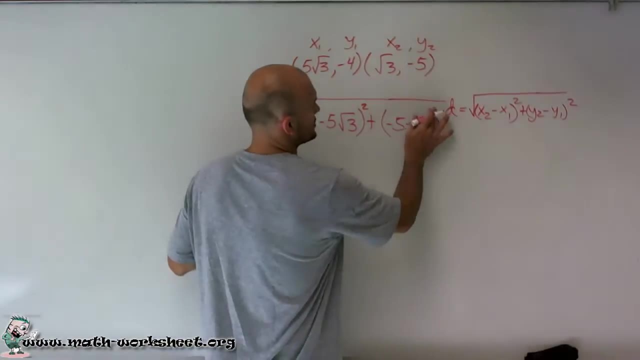 The actual formula is x2 minus x1 squared plus y2 minus y1 squared. So make sure we got that. Okay, just a little mental lapse by me. Then the other thing to make sure is x2 minus x1 and y2 minus y1.. 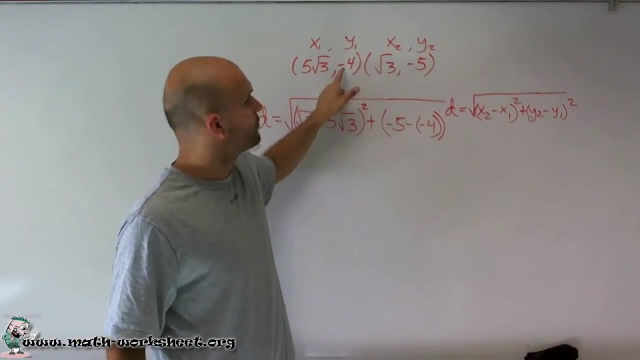 So here I had y2, and then I had minus the y1. You've got to make sure you put those in parentheses. A lot of students will not put them in parentheses and they'll just do negative 5 minus 4.. 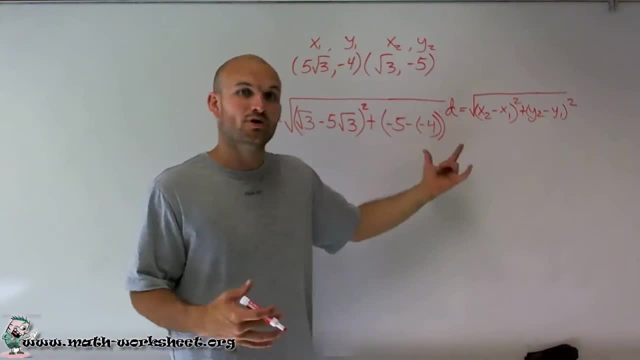 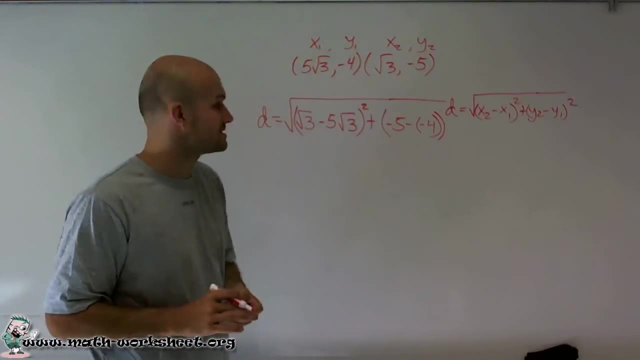 We've got to make sure that it's minus a negative, So put them in other parentheses just to make sure. So here what we have is square root of 3 minus, so it would pretty much be the same thing as just kind of like 1 minus 5,. 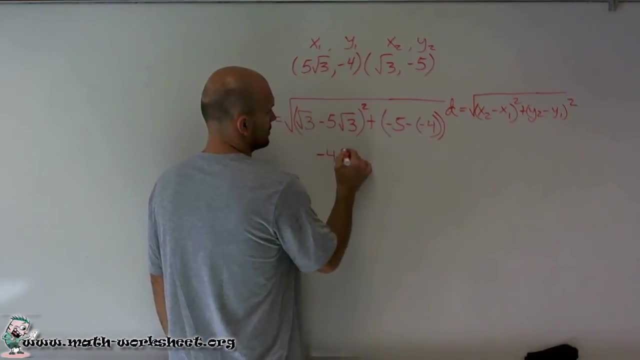 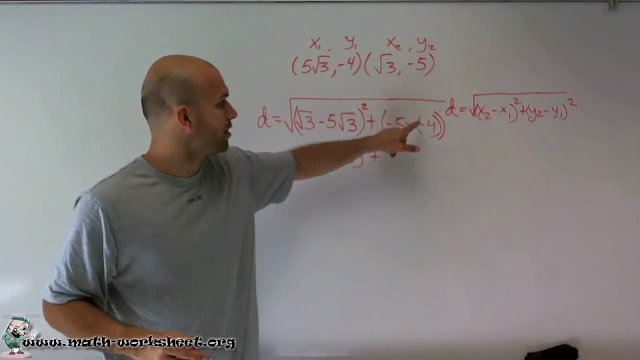 which is going to be a negative 4.. Square root of 3 squared plus negative 5 plus a negative 4.. Well, I'm sorry, negative 5 minus a negative 4, that's a double negative. It's going to turn to a positive 4.. 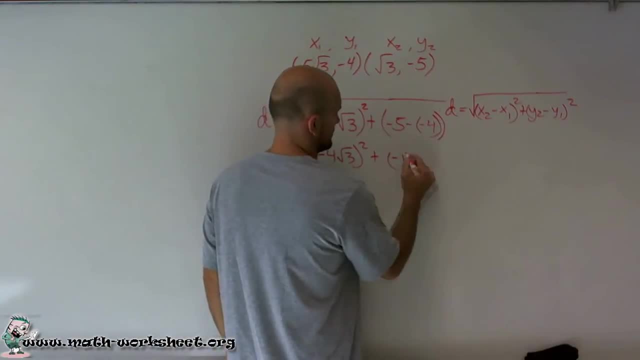 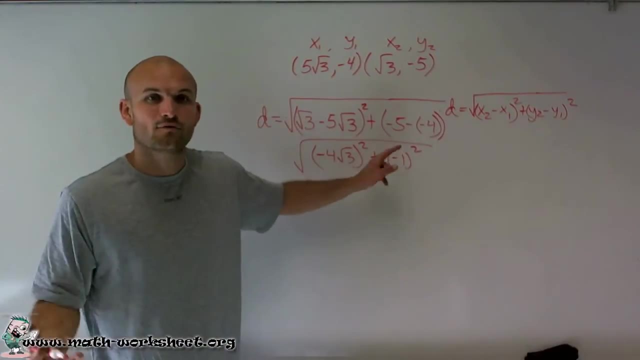 Negative 5 plus 4 is a negative 1 squared, And all of this is square root. So now I just need to square this. Well, this one's pretty easy: Negative 1 times. remember, squaring means that number multiplied by itself. 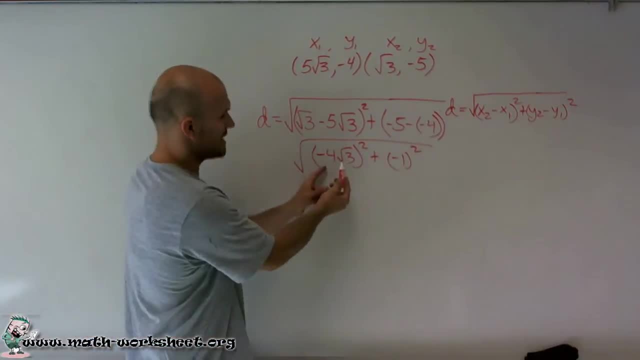 Negative 1 times negative 1 is obviously just going to be 1.. Now, negative 4 times square root of 3 times negative 4 times square root of 3,. what we're going to have to do is multiply the negative 4,.